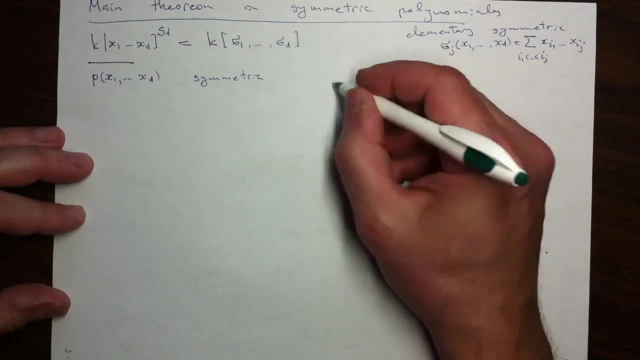 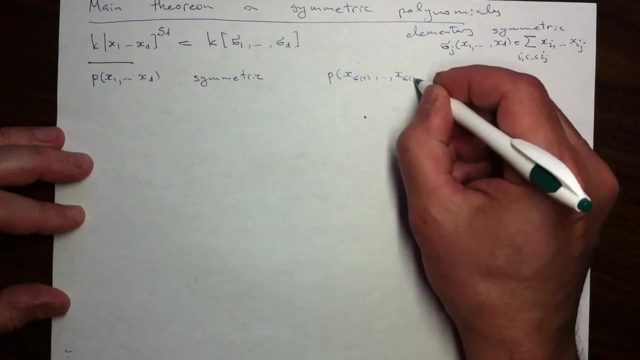 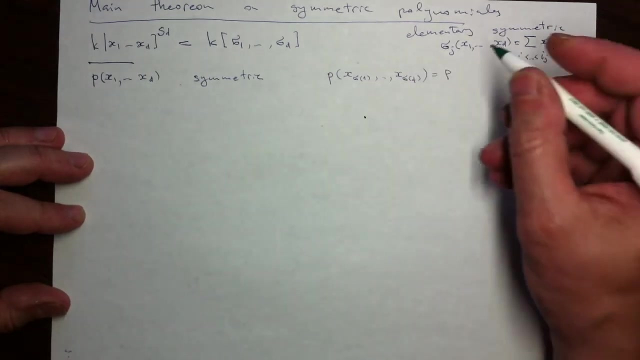 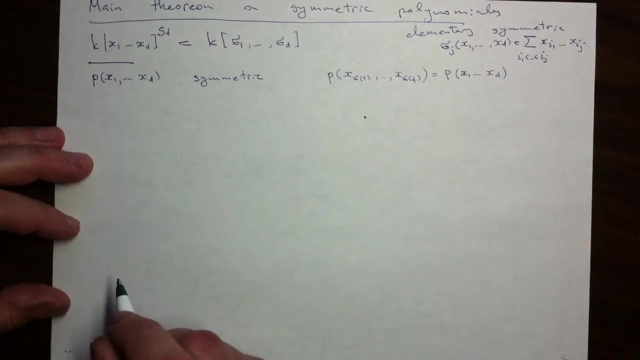 which is symmetric. Again, that is literally that for any possible permutation we can think about. If we do that and put them in places of the original variables, the result will be the same as the original polynomial. it will not feel the difference. So the first reduction: 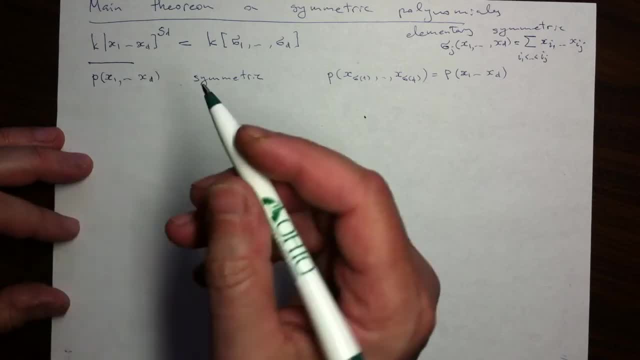 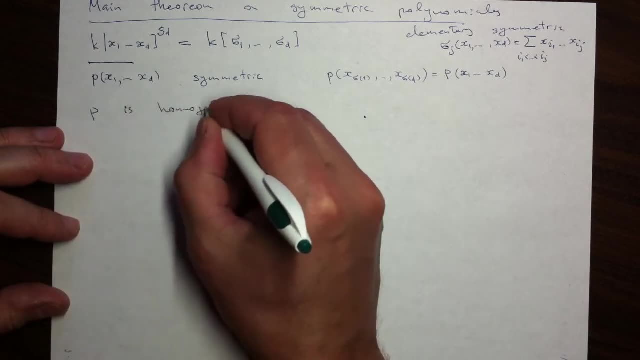 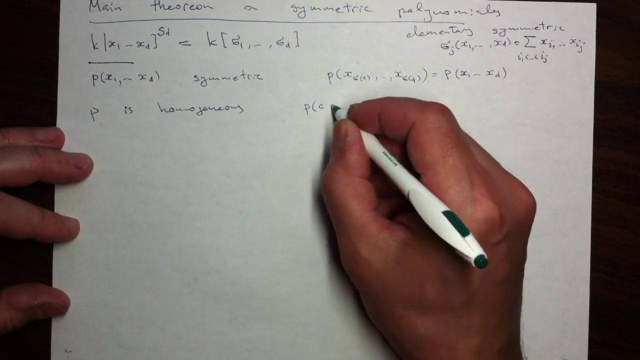 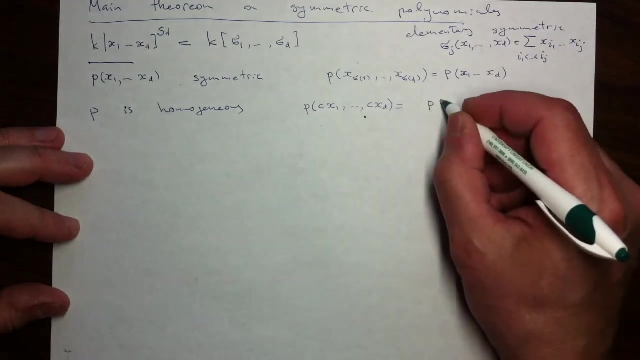 is to break an arbitrary symmetric into homogeneous bits. So what is a homogeneous? A neat way of saying it is to use this functional equation. So let's take our variables and scale them up. V is the same scaling coefficient, O And a homogeneous polynomial will change. 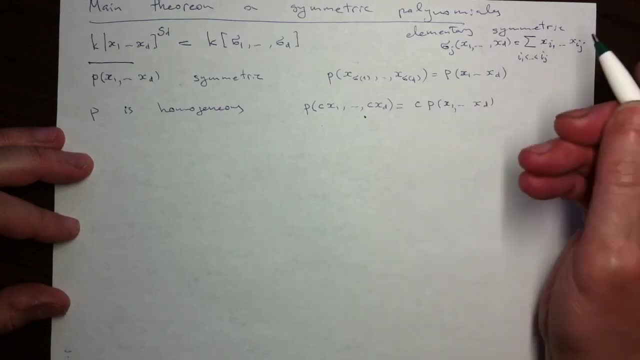 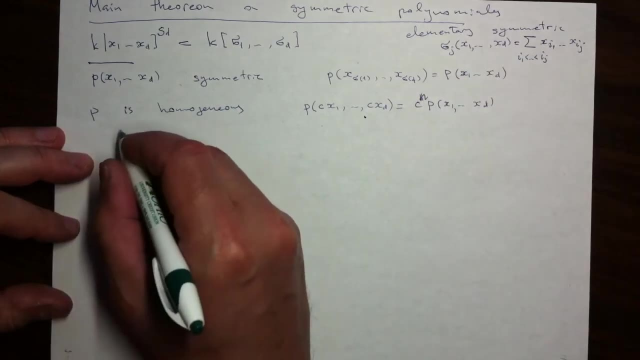 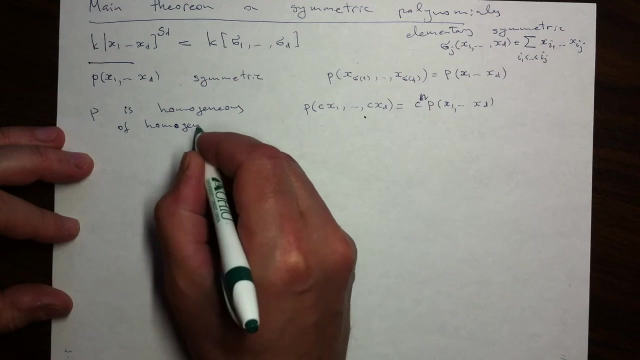 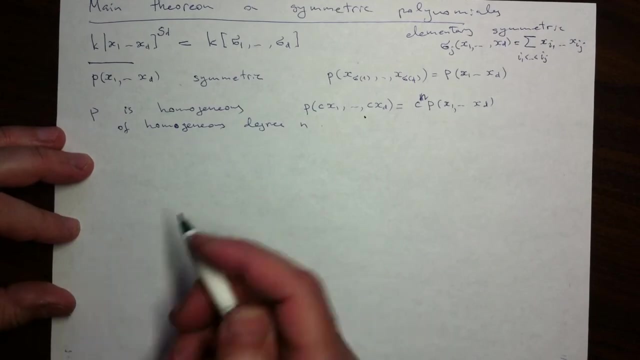 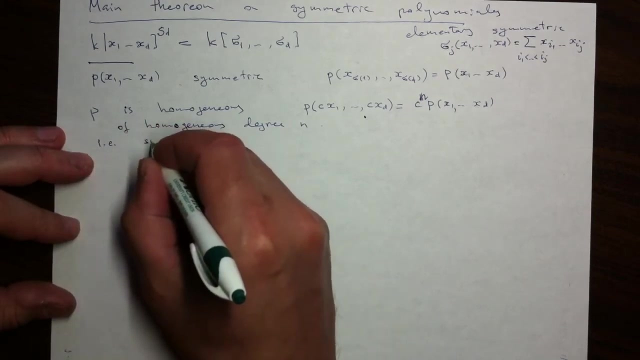 in a very predictable way. under such a transformation You will just acquire a scaling coefficient O, not the same d, an arbitrary m. So that is a homogeneous of homogeneous n, And what it means really down to earth in terms of monomials is that it is a sum. 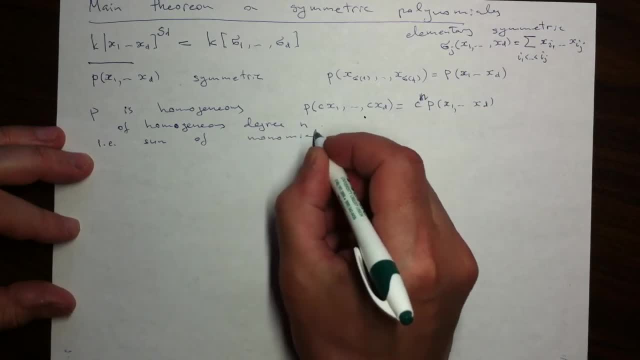 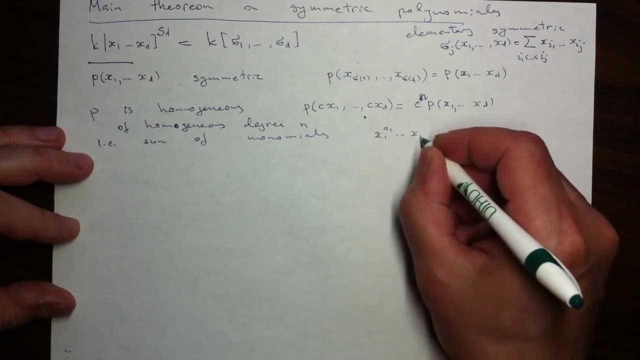 of monomials with some coefficients, but the monomials will have to be with the property that they combined. So that is a homogeneous polynomial. V is the same scaling coefficient, O, And a homogeneous polynomial will have to be with the property that they combined. 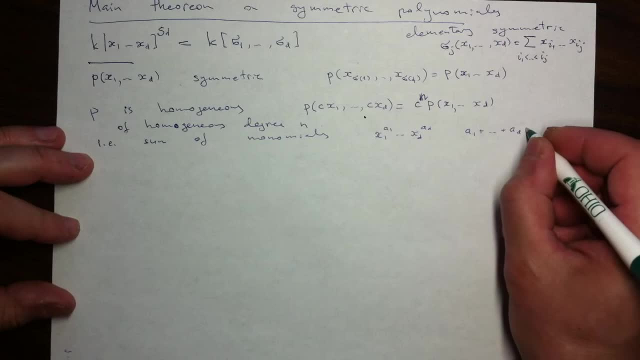 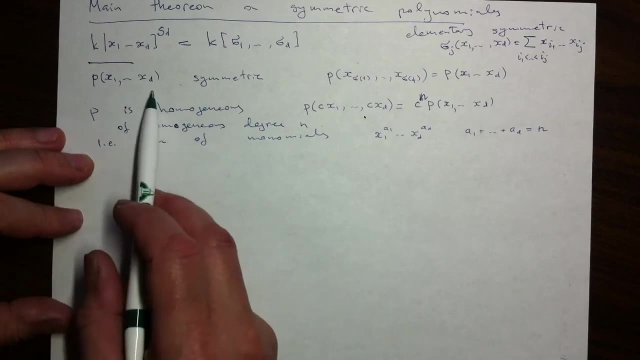 So that is a homogeneous polynomial. So the power of all the variables, the sum of all these powers is n, And we obviously have this property in y-sub-y. So any polynomial is uniquely. any polynomial full stop, symmetric, of nodes, is uniquely. 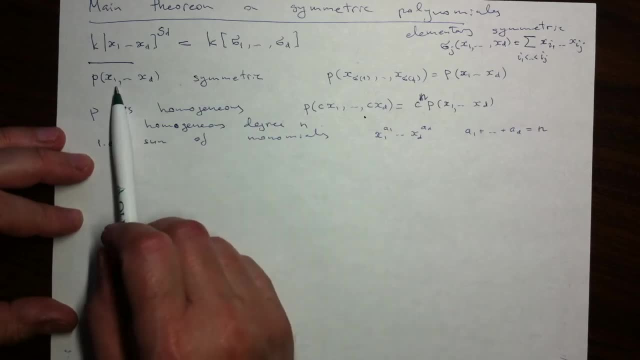 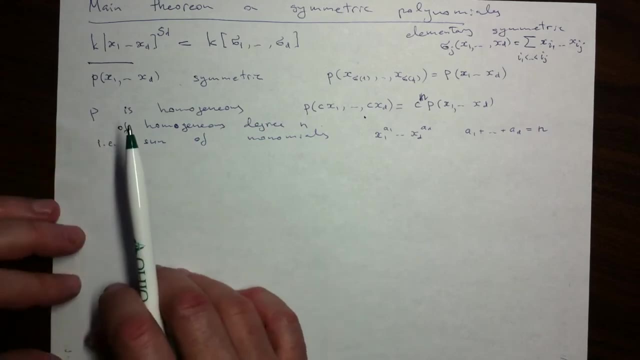 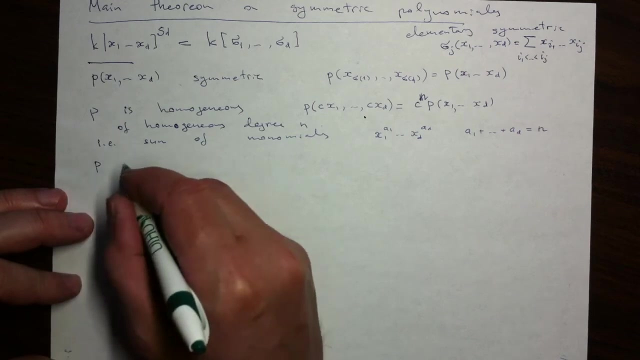 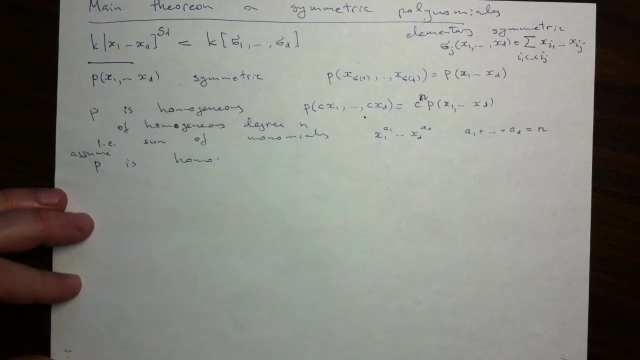 a sum of homogeneous polynomials, And then a symmetric polynomial will have its homogeneous components also symmetric. So that is a reduction to homogeneous case only. So let us assume that p is homogeneous. Now we assume it in the proof And just let's acknowledge the fact that all elementary symmetric polynomials are homogeneous. 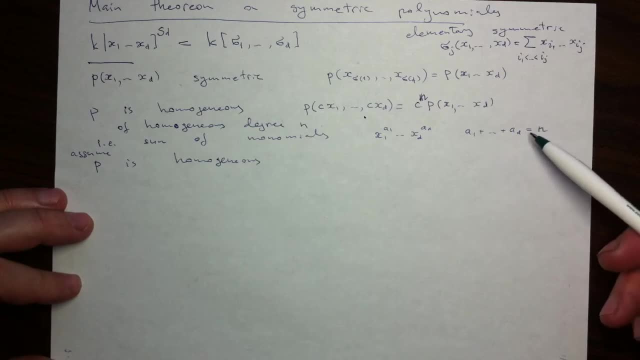 And homogeneous polynomials multiplied and added will give us something homogeneous. So we will always have homogeneous polynomials doing algebraic operations with homogeneous polynomials. So now is the true argument, the body of the argument. We're going to do the induction step by decreasing certain more fine order than the homogeneous. 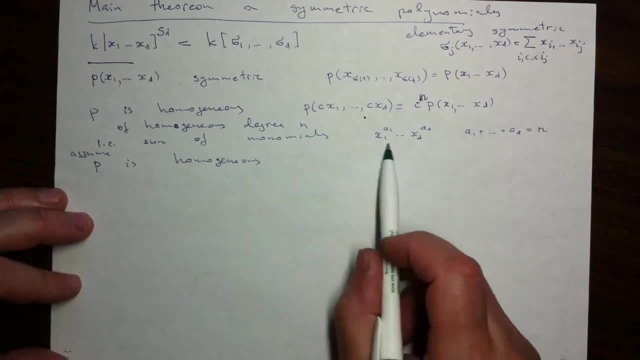 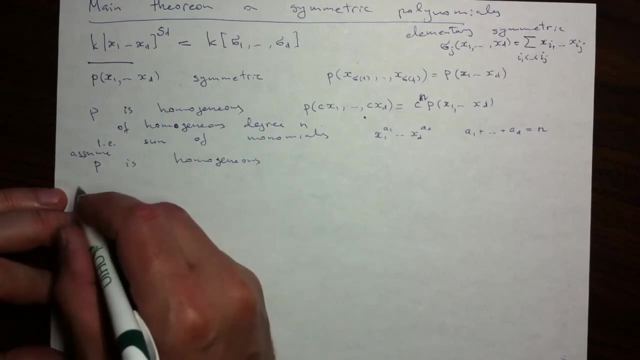 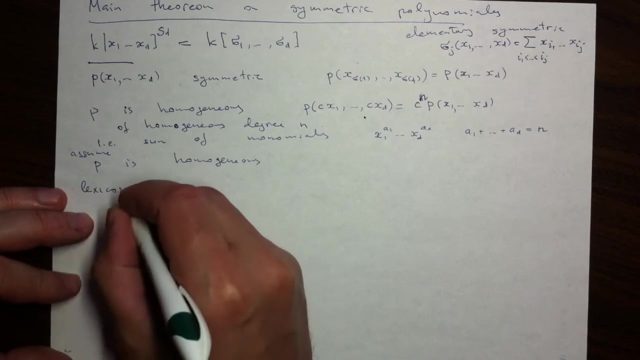 degree. And that is the order on monomials, and that is a perfect order. so all of them will be linearly ordered. So let's just do this definition First. the lexicographic it's called introduces a perfect way of ordering all monomials. 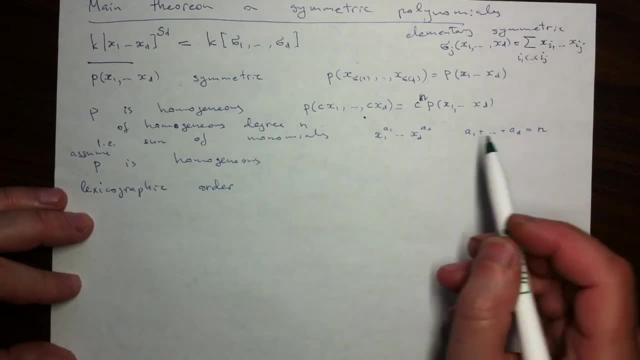 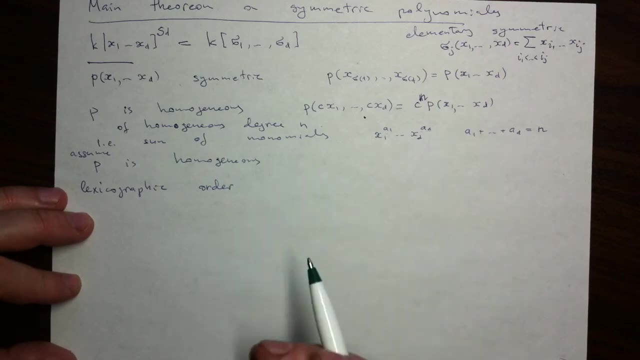 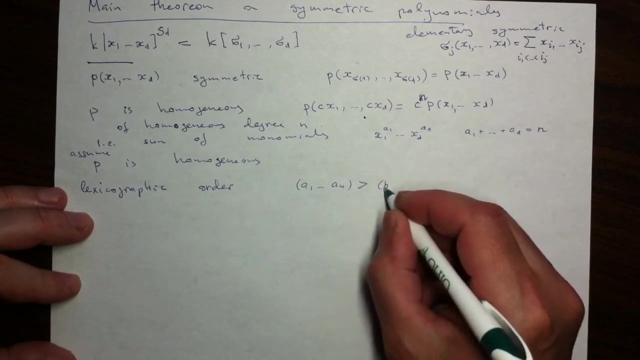 And it's really a way of ordering important information about monomials, collections of powers, Cost' co-ordinates, Natural number co-ordinates. So we just say that this vector whose co-ordinates A-s and its larger than the vector whose 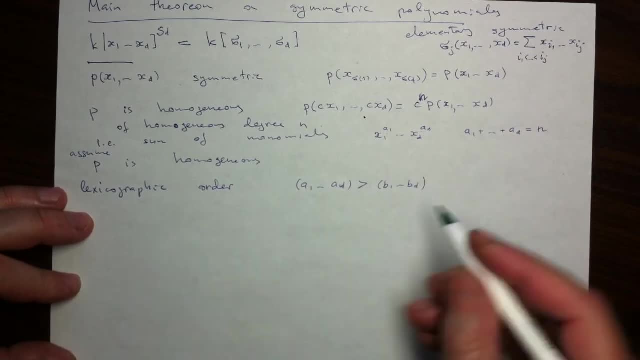 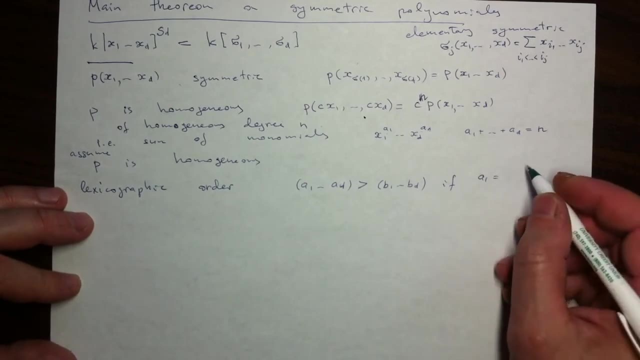 coord-inates B-s have to have x-coordinates. If either, Well, I will write a general situation. So I'm comparing two vectors, I'm comparing the first coordinate. If the first coordinate is larger, then the first coordinate is bigger. 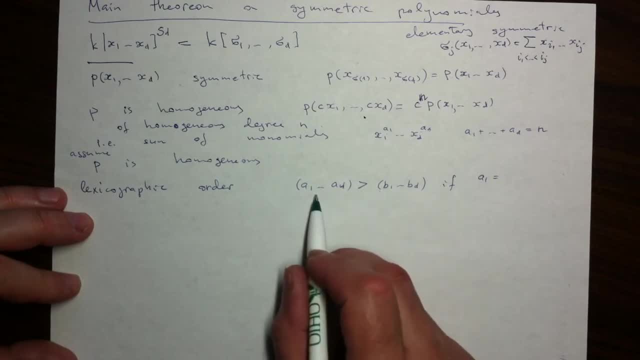 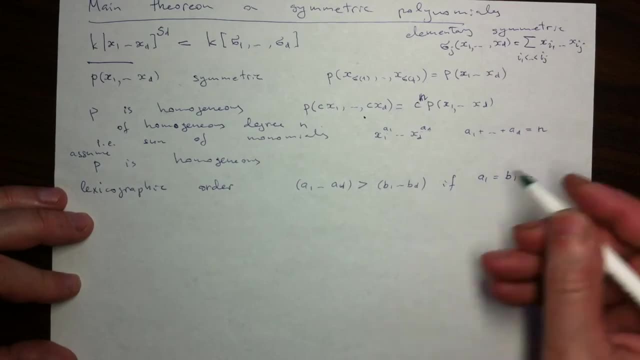 And the second coordinate is smaller Today, I agree regering of coordinates vector- then the first vector is declared to be larger If they're the same. I'm comparing the second coordinates and then I'm comparing them till they stop being the same. So 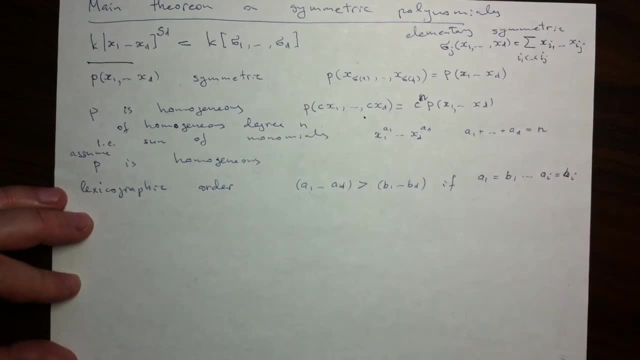 say: I'm going, we're seeing the same coordinates till position i and then at position next, i plus one, I should have this inequality And then this vector is declared to be larger than this. So again, the process of comparison is: we start with the first coordinate, we compare them. 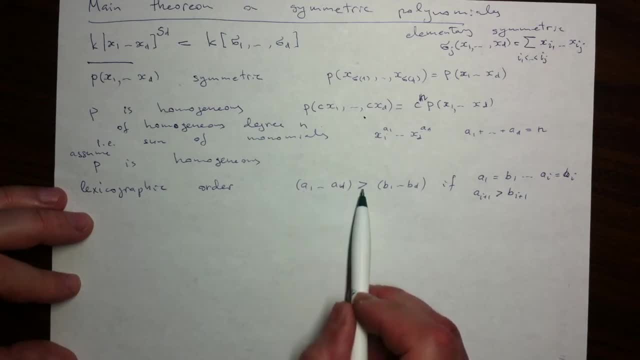 If they are in this inequality, then we're fine. If they're equal, we'll proceed to the second and continue. So that is this lexicographic order which puts in a string all possible vectors of powers, hence all possible monomials. 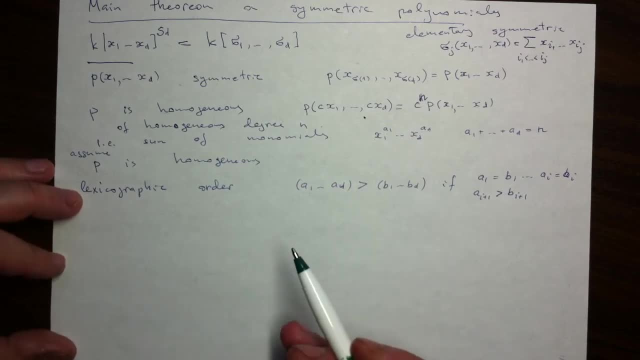 So the induction will be on the highest such monomial. Let's now employ the condition that our polynomials are symmetric. So the highest monomial of a symmetric is a polynomial p. Let's record this co of the efficiency, the powers of the variables And then the condition which is inevitable from. 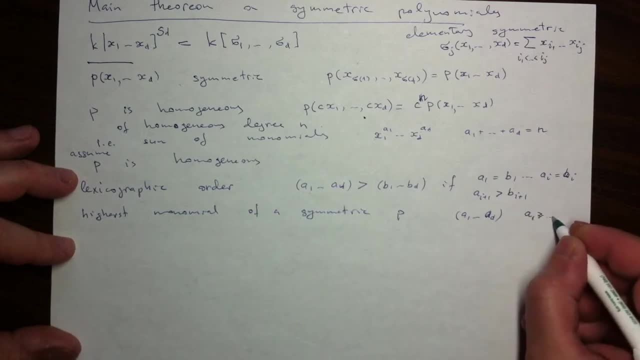 the symmetry property is that this sequence of natural numbers of these powers will have to be non-increasing, So the first should not be smaller than the second, and so on. Well, it's simply because of the symmetry of our polynomial, we can change the order of our variables. 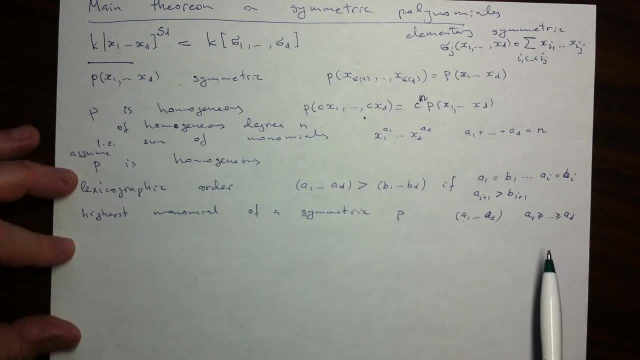 but we can also permute the coordinates in an arbitrary permutation way. So here I should add the quantify for all permutations, And permuting a coordinate vector with arbitrary permutation, I can always make the first coordinate to be the largest of all and the second coordinate to be the 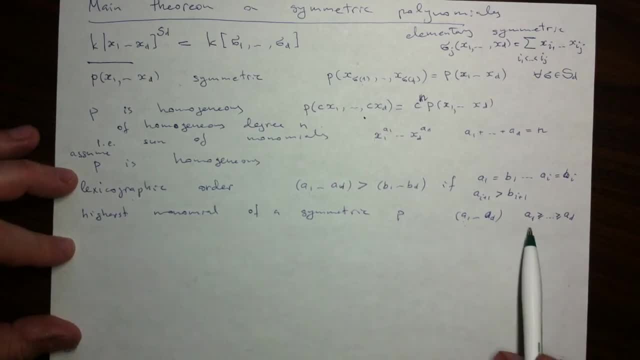 largest of all remaining, and so on, And in my lexicographic order it will be larger than anything else. That's why the highest monomial of a symmetric polynomial will have to have this property. We could look at what the elementary symmetric polynomials have as their highest monomials. 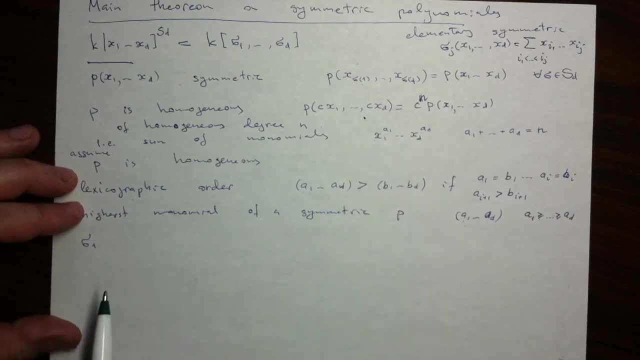 or highest vectors of powers. So in sigma1, this polynomial is just the sum of all monomials, and the highest monomial among these is the first one, and the vector will be 1 and all zeros. Sigma2 is the sum of all products of two vectors. 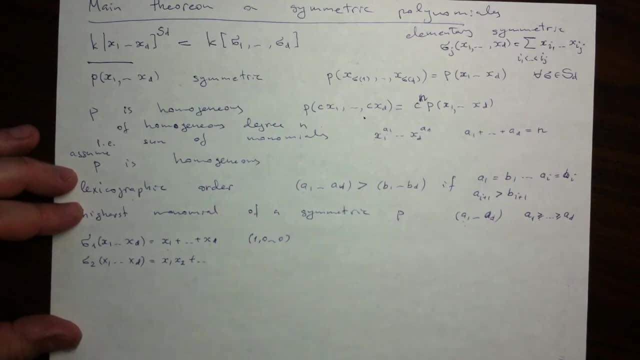 And the highest of such products will be x1 and then x2, and the vector of powers will be 1,. 1 and then zeros, And all the way down to the very last number, d I will have for the very last symmetric. 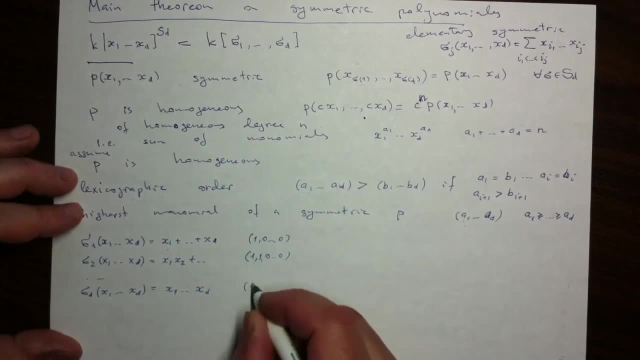 I will have just the product of the variables and of course, the product of the variables And the vector of the powers is just all 1s. So these are the vectors, the highest vectors of our elementary symmetric polynomials. What are we going to do now? 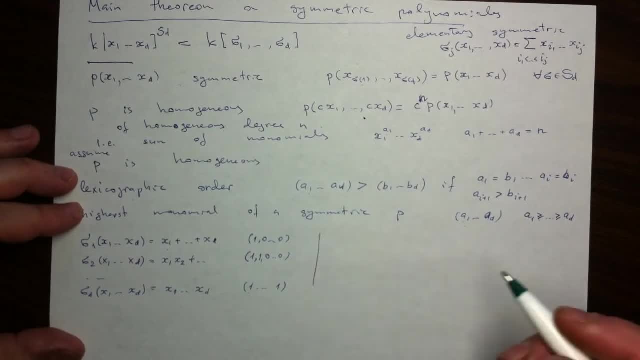 We are going to run the induction step. So we are going to start with a polynomial, take its highest vector and use this property to match this highest vector with the highest vector in the product of elementary symmetric polynomials. So we just need to combine these elementary symmetric polynomials. 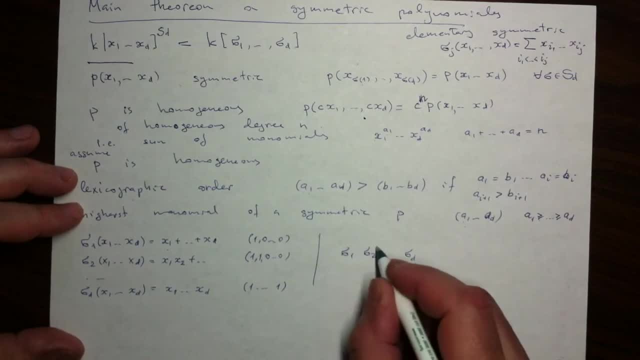 Take the highest vector. Take the highest vector. Take them in some combination of some powers, take the product of them and make it such that the highest vector will be this. And that is easy, because computing the highest vector in the product is just adding these. 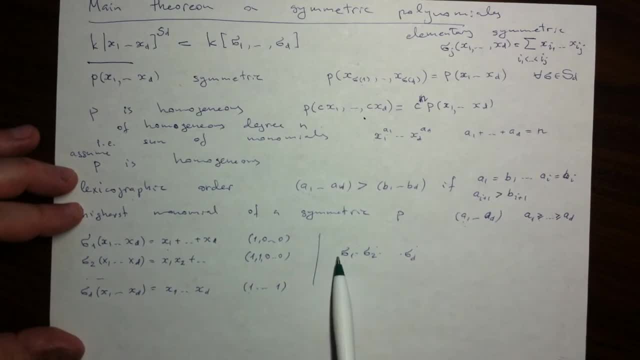 vectors of powers. After all, the highest monominal here will have to be multiplied with the highest monominal here. with the highest monominal here, if they come with powers, then these highest monominal will have to be raised to those powers first. 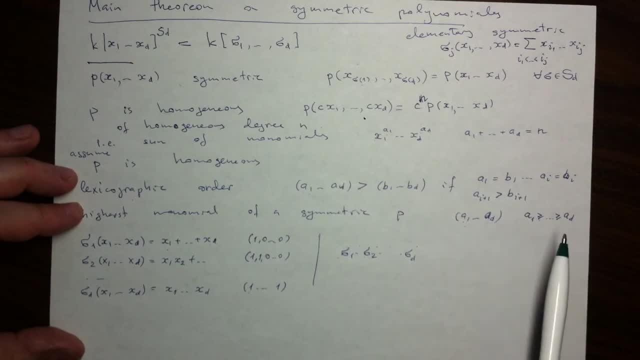 And that is all neatly expressible in terms of the vectors. We just need to add these vectors. That's what happens when we multiply the corresponding monomials. So we'll have to measure the power here and the power here and all the way down to the. 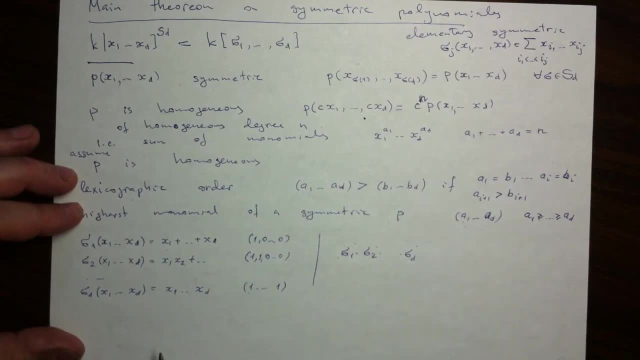 very last, powers, such that the highest vectors with these coefficients will match with this vector. And I will just write you the answer And you please check that this is correct. Thank you, Hopefully it works. So the first power will be the difference of the first coordinate and the second. 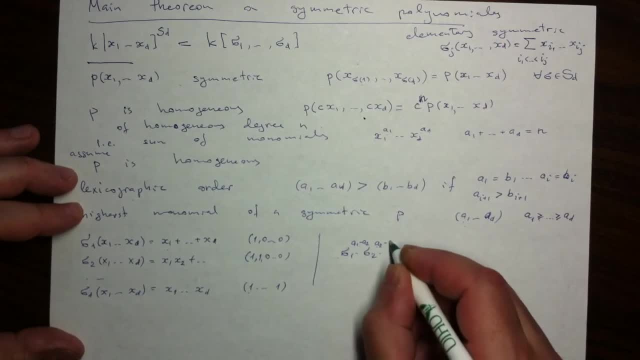 The second power for sigma 2 will be the difference of a2 and a3, and so all the way down to the very last, And the very last will be the difference of ad, and nothing after. make it zero, So that monomial in elementary symmetric polynomials will have the highest vector, just as our polynomial. 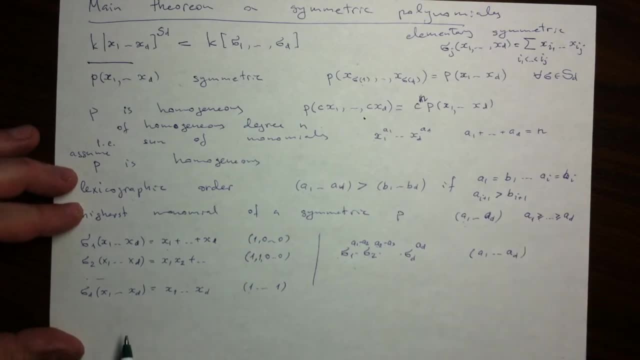 p, This given a1 to ad. And now, if we take the difference of our given p and this expression, this monomial in sigmas, its highest term will be smaller, Smaller in this lexicographic order And that is the induction step. we make it smaller and we cannot go forever making it. 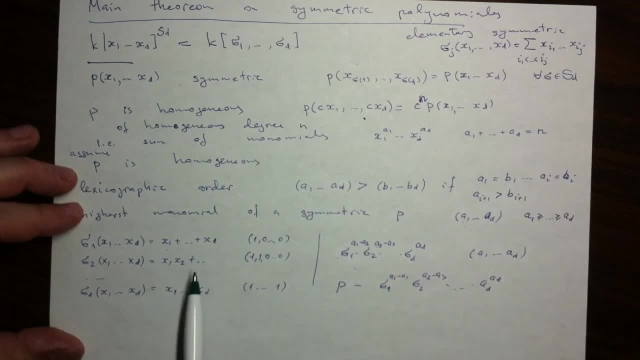 smaller, Because there is only finite number of vectors which are less than the given one. So we will have to stop sooner or later. And that is the proof, by induction, that any symmetric polynomial is a combination of elementary symmetric polynomials And the uniqueness comes from the construction, because at every step we are determined. 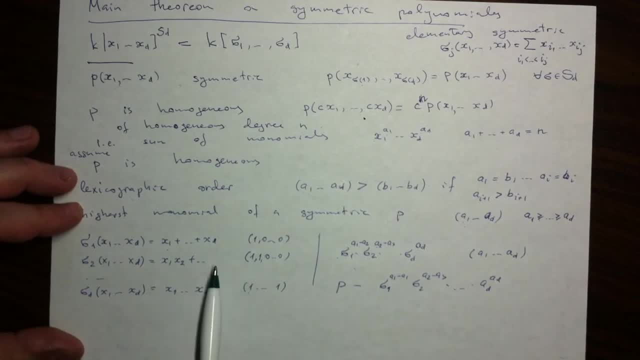 What we have to take is completely determined by this equation, And so the result is completely determined. Let me finish by looking at the example. So let me take something easy, as my input is just symmetric. so we will have, say, three variables, x1, x2, x3- and I will cube them and take the sum. 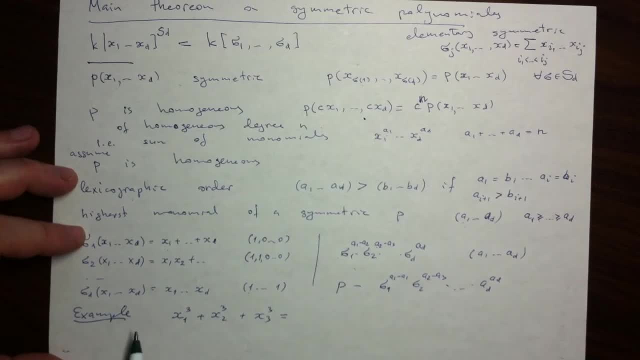 That makes it symmetric. So that is supposed to be an expression in a unique way in elementary symmetric polynomials: sigma1, sigma2, sigma3.. So let me write those sigmas. So that is supposed to be an expression in a unique way in elementary symmetric polynomials. 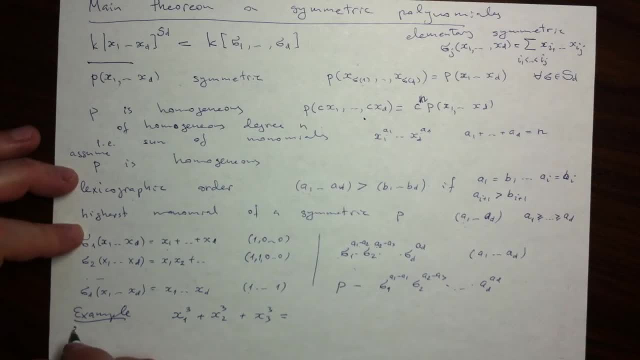 And then sigma1 is again the sum. Sigma2 is a sum of all products: x1,, x2, x1, x3,, x2,, x3 and then sigma3.. Yeah, nice, paar, alph manej container cinco ok. 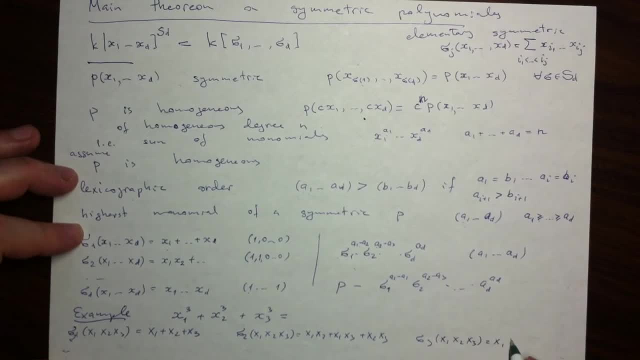 is just a product. So, looking at this, I know that the highest term is the first one and the highest vector of that is 3 and 0 and 0.. And then to create the product of elementary symmetric with the same highest term, well, it's obvious. I. 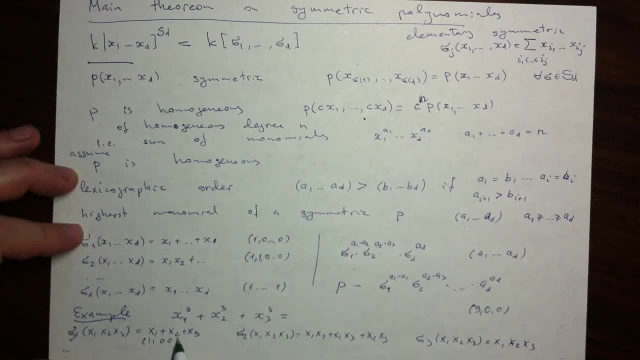 just have to take this one. I just have to take this one, 0, 0 and take it three times. So cube it, sigma 1 cubed, And the coefficient for this is the same as the coefficient in here. Because, again, if I 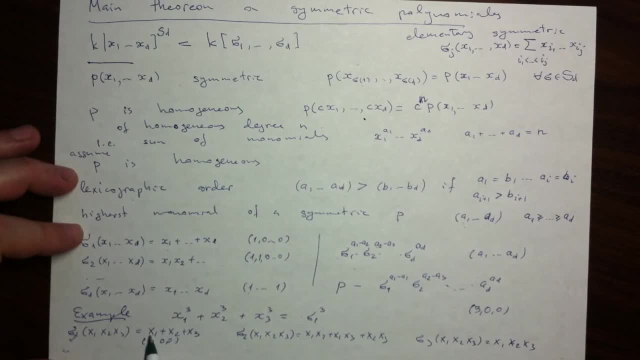 cube my sum. if I cube this sum, my leading term will be x1 cubed, matching perfectly with this given one. So that is definitely inside the expression. Instead of doing induction as in the proof, we could really kind of imagine how it's supposed to. 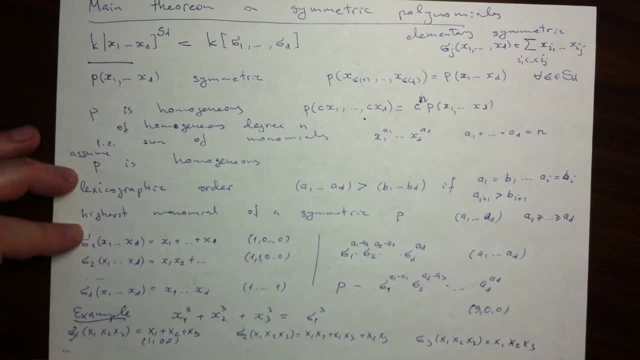 unravel And other terms, other products of elementary symmetric polynomials will have to have their leading terms not larger than this one, but actually smaller. So let's list all possible vectors which are smaller than this, But they have still to be. they still have to be. 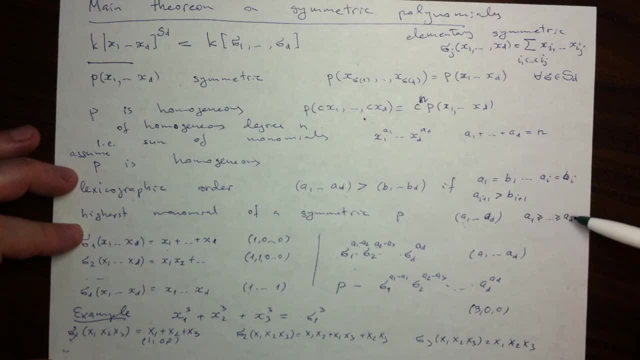 subject to this condition: They have to have coordinates forming a non-decreasing, non-increasing sequence. So the next, after the 3, 0, 0, will be 2, 1, 0.. What, effectively, I'm doing? I'm taking one of. 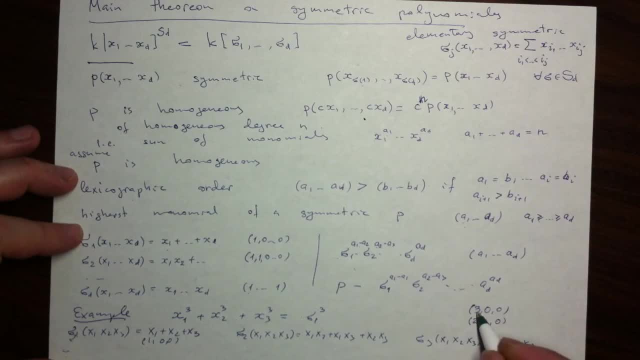 those ones and moving them to the left, to the right, sorry, And I should really not make gaps because, again, it should be non-increasing at every step, And the one after will be 1 and 1 and 1, and that is it. you can see. 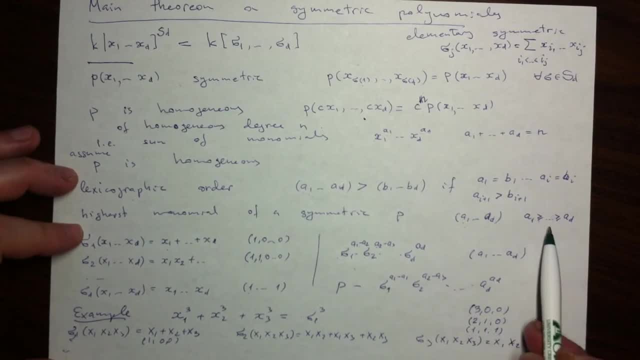 that no other vectors will be non- increasing and in sum equal to 3 and then lexicographically less than the given one. And now I have to imagine what are the products of elementary symmetric with these leading monomials. and for this one, 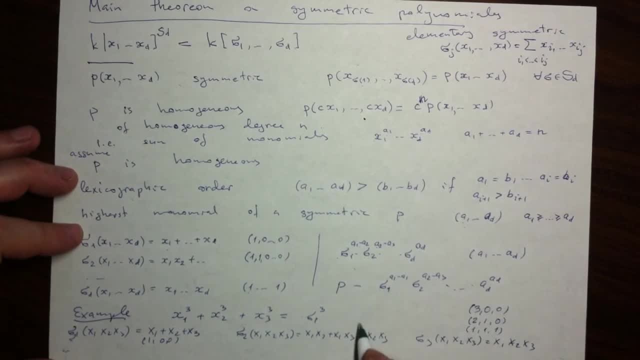 again, that is a recipe. I take 2 minus 1 and that is just the first power of Sigma 1.. I take 1 minus 0 and that is the first power of Sigma 2 and then 0th power of Sigma 3, so it is not present And now I'm not seeing immediately what the 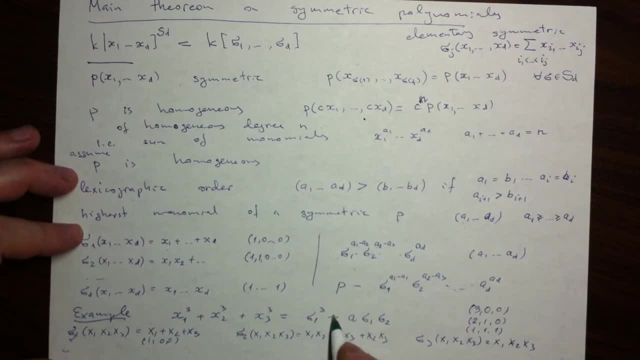 coefficient is. so I'll just introduce some parameter a here, And then the very last vector will correspond to Sigma 3. so that is really the leading monomial, the only monomial in Sigma 3.. So Sigma 3 is also in the expression, with some 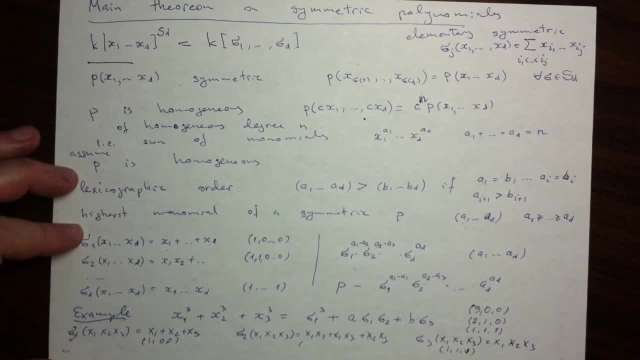 unknown coefficient b. And then to find this coefficient, here is a useful trick. We could look at a function of the equation and then evaluate it at some specific values for x1,, x2, x3. And this way we can see what a and b have to be. So my first. 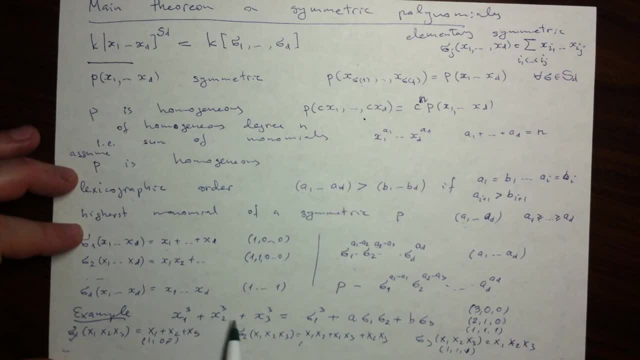 evaluation would be to evaluate on the collection of 1 and 1 and 0. So, evaluating at the variables 1, 1 and 0, my left hand side will be equal to 2.. On the right I will have Sigma 1 on so and. 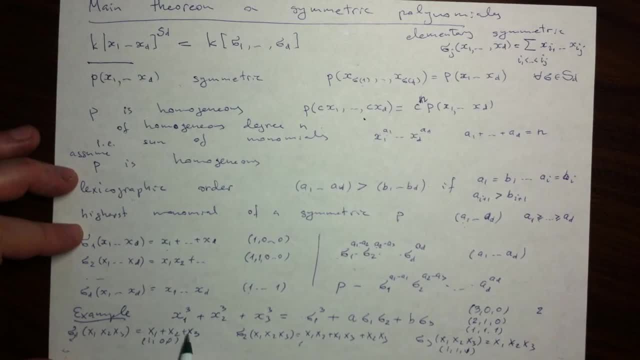 one zero makes sigma one to be two, so that is on other side two, but two is to be cubed and then sigma one again is two and sigma two on one. one zero will be just one and one and then all the other two. all the other two terms are zero. so that will be just one and that is with. 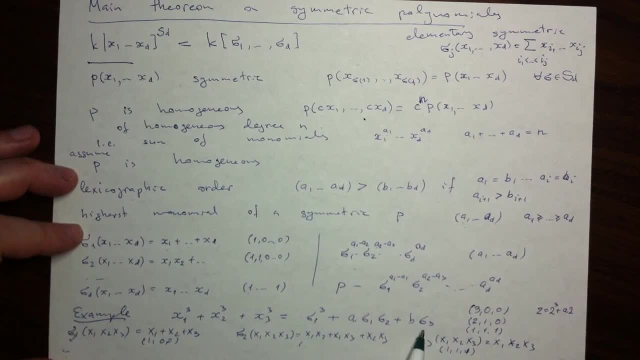 coefficient a and then sigma 3 is the product of 1 and 1 and 0 into 0. so this is just an equation for a which, after you do the constellations and all that, gives you the answer negative 3.. and then you can find b by again evaluating on a different collection of values for x, 1, x, 2, x 3. 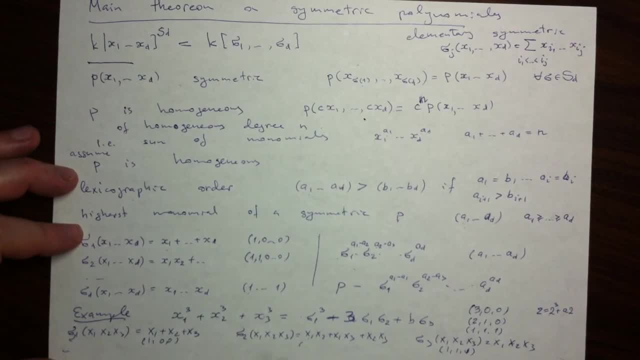 so you take 1, 1 and 1, then on the left you will have 3 and Sigma 1 will again be 3 on this connection, so it will be 3 cubed and then Sigma 1 will be 3, so you have 3 squared and Sigma 2 will be 3. 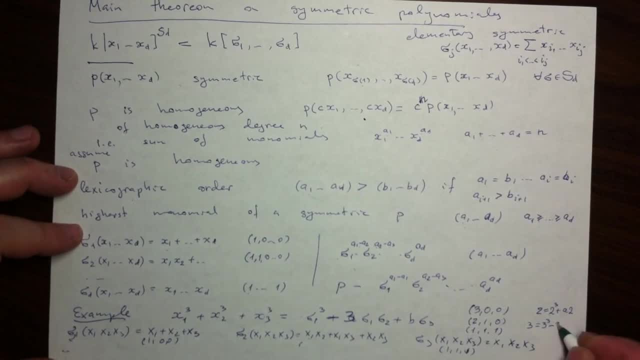 because 1, 1, 1, 1, 1, 1 will give you 3, so you have 3 cubed again with minus sign. and then you have Sigma 3, which on 1 1, 1 will be equal to 1, so you just have your. 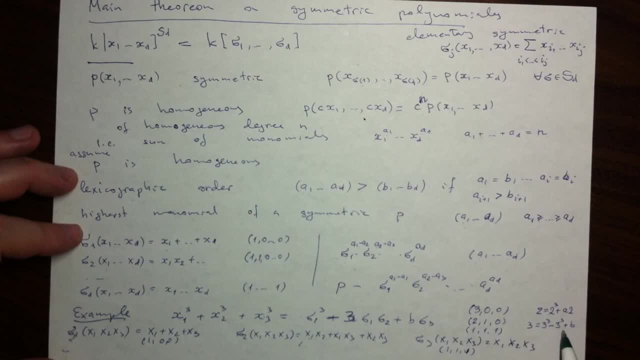 b and that is a perfect answer for b, it is 3. so that is a quicker computation exhibited in this general statement that any symmetric polynomial is a combination, unique way, combination of elementary symmetric polynomials of some coefficients. so you could check it by plugging back what Sigma 1 is. it is a. 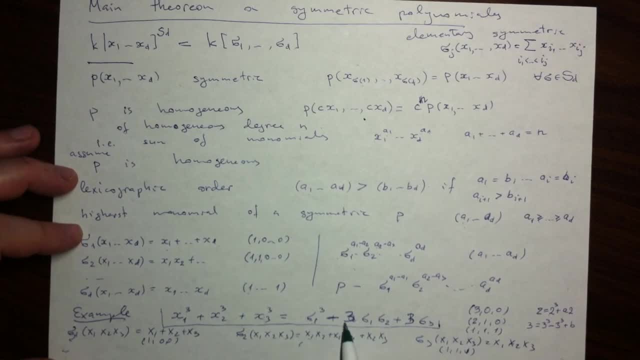 sum of all axis cubed. then here you have, with coefficient negative negative three, the sum of all the variables times the sum of all products of pairs of variables, and then you add three copies of just the product of all the three variables. so that is one example of this main theorem on symmetric polynomials. 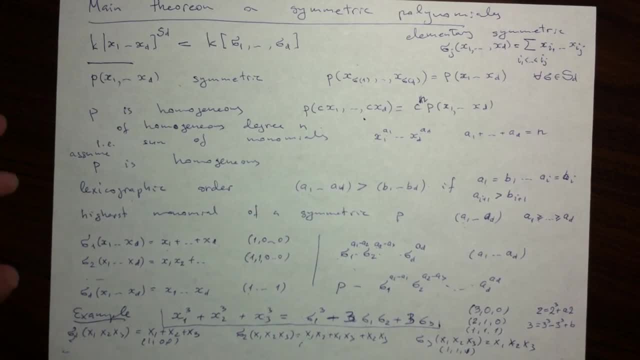 more are to come. see you later. 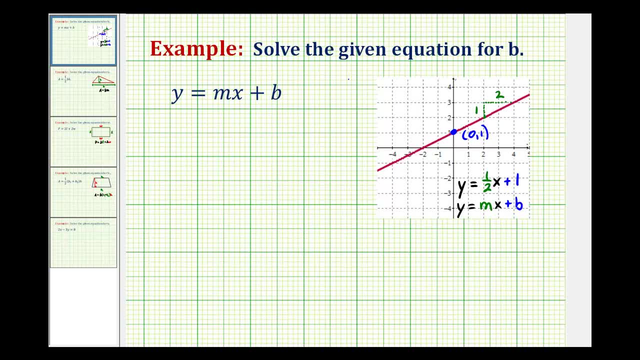 In these examples, we'll be given an equation or a formula and asked to solve the equation or formula for a specific variable. While this might feel a little bit strange, we're just really practicing the procedures that we use to solve equations, And one of the main things to remember is that, whatever we do to one side of the 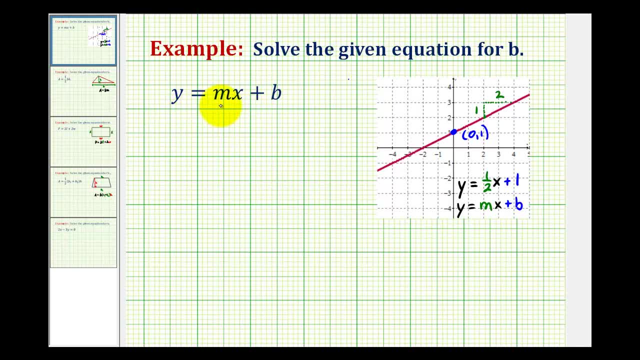 equation. we must also do the same to the other side of the equation to maintain equality. So here we're, given the equation: y equals mx plus b, which happens to be the slope intercept form of a line, as we see here on the right. But the goal of this problem is to solve for the variable b. 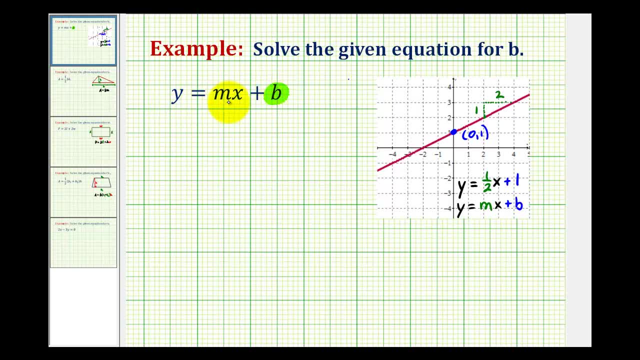 So even though y and mx are variables, we'll treat them as constants in order to isolate b. What I mean by that is if you can solve an equation like this, let's say five equals two plus x, then you should also be able to solve y equals mx plus b. for b To solve this one step equation, we would just subtract: